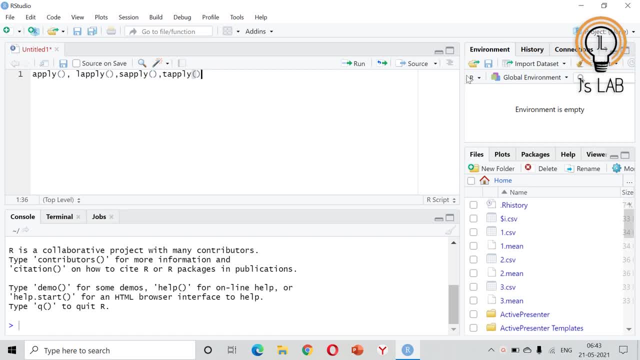 be very useful and handy. So these are the apply functions. That means first of all, apply, l apply s apply and t apply For dealing with data processing, data analysis. this will be very helpful for you. First we will study about apply, then l apply s apply, and. 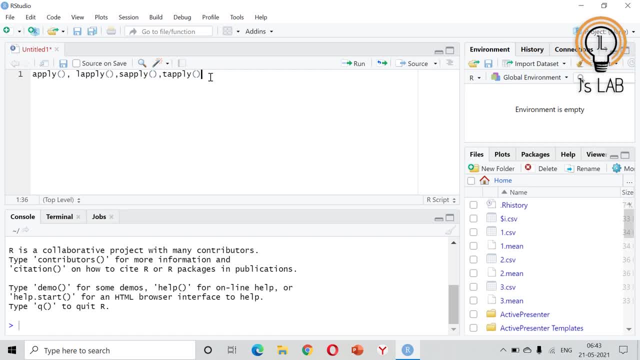 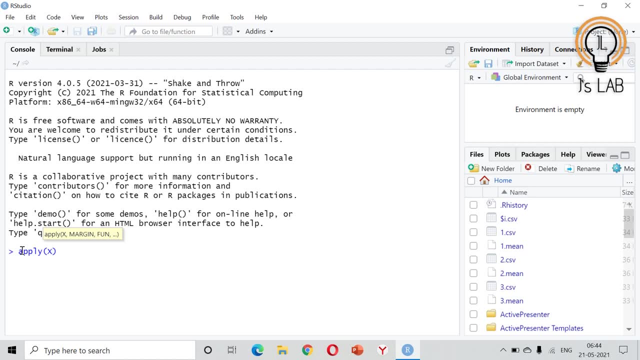 t apply with examples. So we will start with apply. So I will remove this one First. we will start with apply function. Apply function. this is its. So in this arguments, you need to provide a margin and a function. You need to do So. 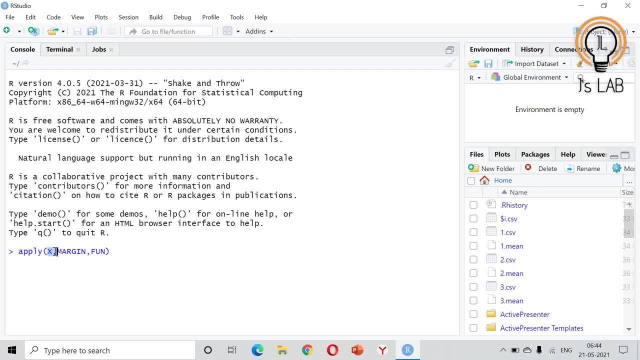 this is the general. So in this x means that is the value that you need to give, That means it might be a matrix, it will be a vector, etc. And margin: it takes two values: 1 and 2.. Margin equal to 1 means it manipulates on rows and margin equal to 2 means columns. 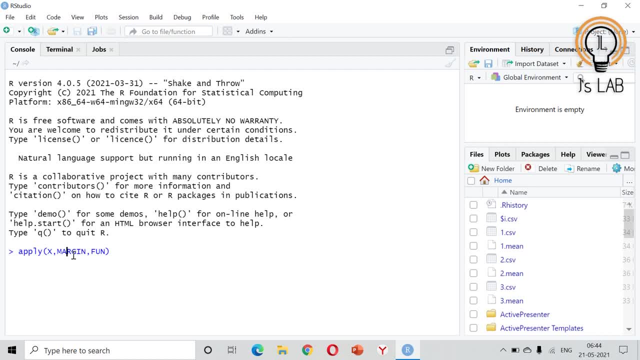 And margin equal to 1 means it manipulates on rows and margin equal to 2 means columns And functions means which function you need to apply. For example, you need to find the sum median or your own function, user specified function, etc. So we will see with an example. 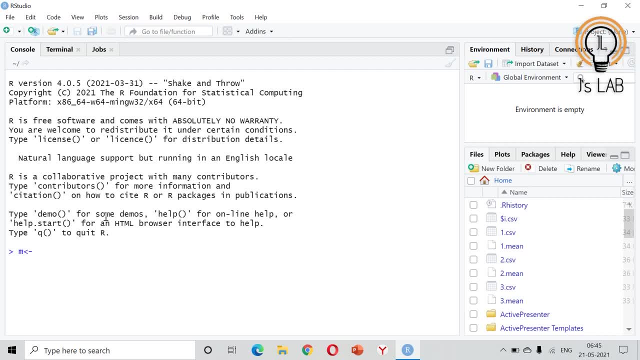 So for that we will create a matrix. We will create a matrix and the values will be from 1 to 10, take from 1 to 10 and number of rows equal to 5 and number of. I am just creating one. 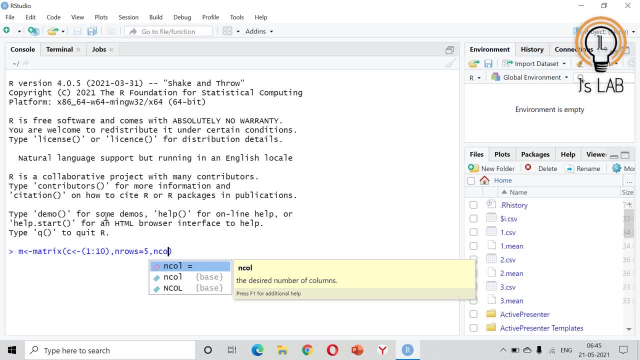 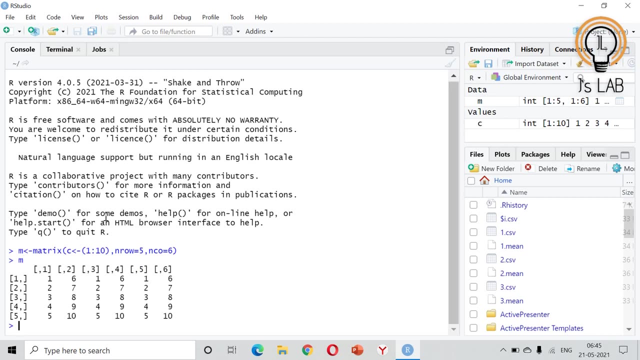 Number of columns n equal to 6.. So there is no rows. n row. Okay, so we will see the matrix. So this is the matrix. So to this matrix we are going to apply the apply function. 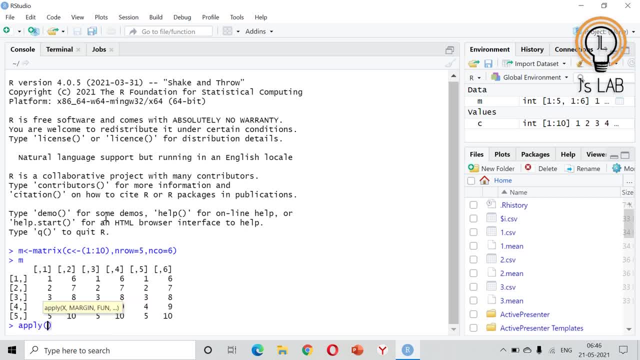 So apply, and first of all, in the place of x, that is the matrix M, Then then we will provide margin a, 2 for example. So 2 represents 4 columns. Okay, so I am dealing with column. 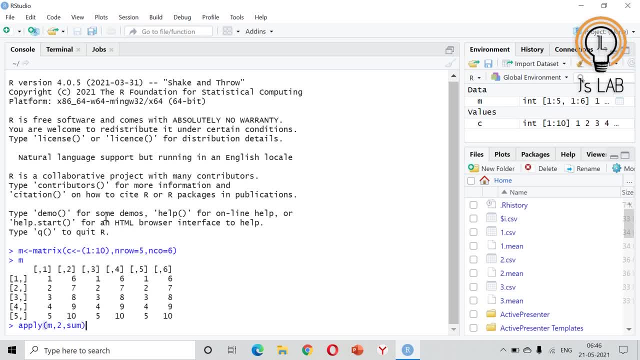 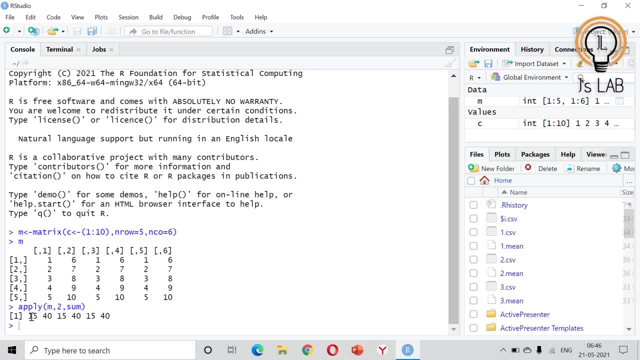 and function. I need a sum, Okay, So if I put that, say, see in each column, see each column, it will calculate the sum and it will be written here. This is the first column sum. second column sum, third column sum, fourth, fifth, sixth column sum: Okay, And 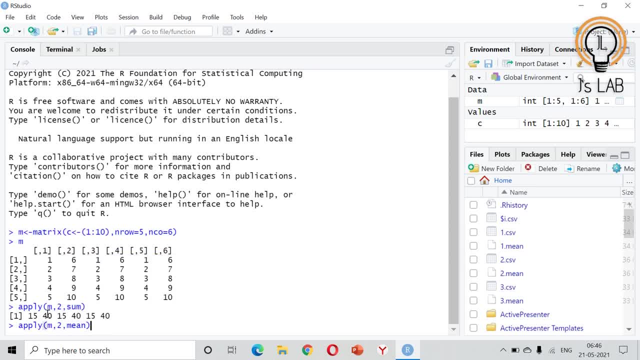 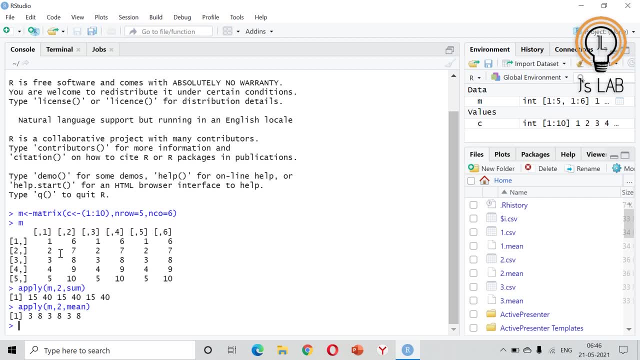 instead of sum you can put mean. I will write here: this is the first column sum, second, third, fourth, fifth and sixth column sum. Okay, And instead of sum you can put mean, mean. So each column mean will be displayed. So that is the apply function. So it takes. 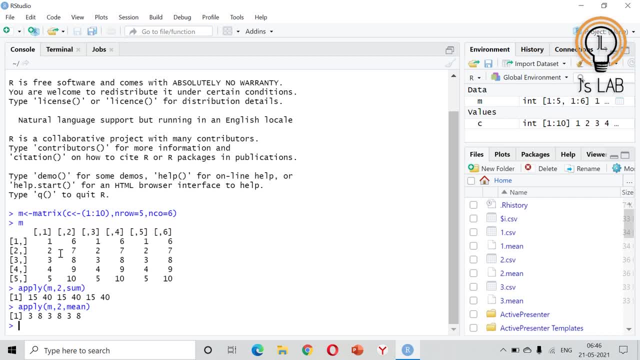 data frame or matrix as an input and gives outputs in vector, list or array. Here it has taken the matrix and given as a list. So that is the apply function. Now we will see L apply function In L apply. I will use this one to explain just a script: L apply function. 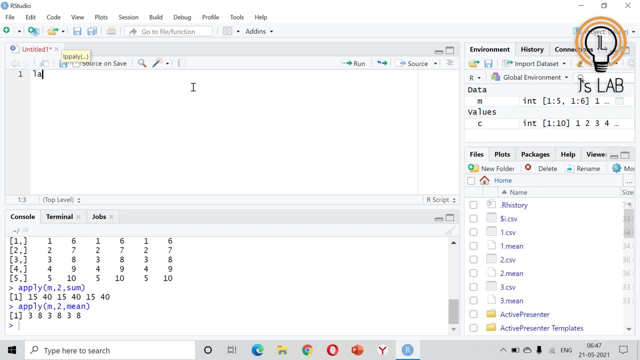 L apply function is the L apply function. L apply function will not take margin. do not require margin. It requires x, and x means that is the input, whether it is a vector list or etc. And that is the function, is that you need to perform. So x is a vector or an object. 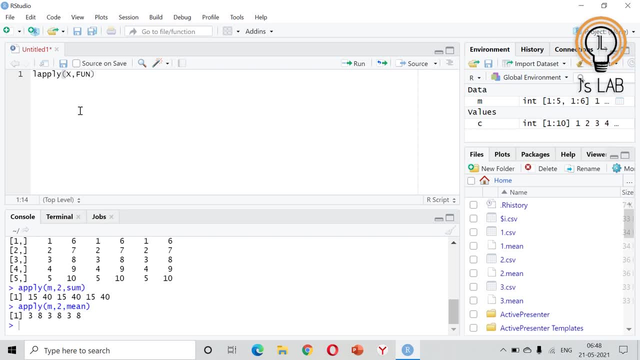 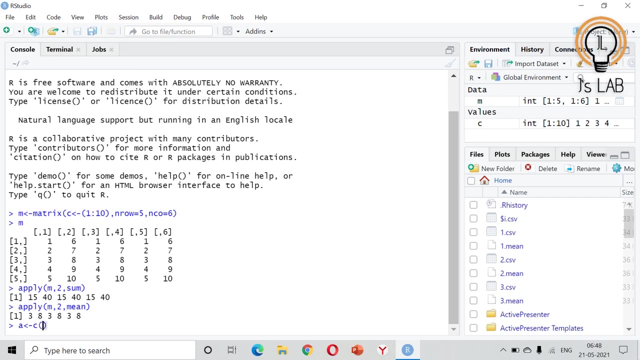 and function means it is a function that you need to apply on each element of x. So we will see an example. Remove this one and we will move back to the console. So we created a. we are going to create a vector of some names, characters in capital letters. So 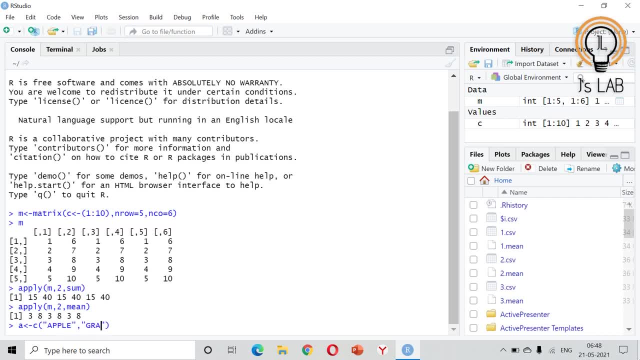 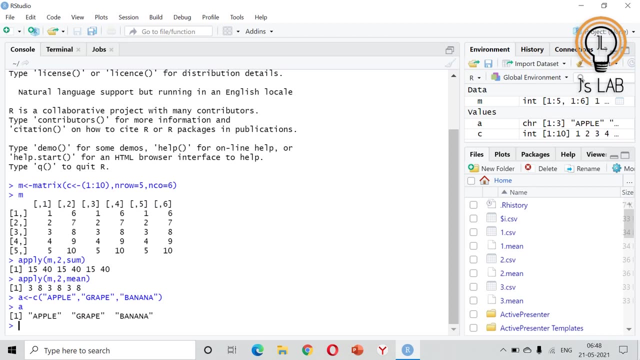 tickr apple grape banana. Let us create it. We will weird that one, sorry. So it has been created. Okay, Now we will apply. L apply and I want to change all the letters. So this is the x means input to the L apply. I need to change the upper case. to lower case, Capital letters to small letters. So let me check an row first. Tell me if I know your value in terms of number. What would that be? So let us just sort of plug that two drives in and then add the next to these, Then our two pays, and hence I have therefore in onetag there is the example S, that I have a capital letter. Now we will apply a louder define only if 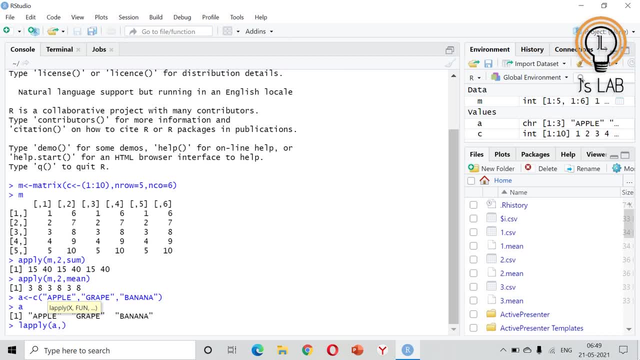 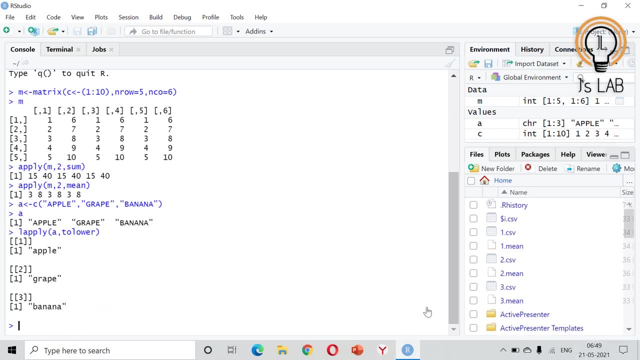 us and apply a- that is our input- and to lower. so everything has been changed to lower- see apple, grape and banana. but this is not a list. so if you want to output in list form, you need to modify this one, use the unlist form, the entire thing inside unlist and see now. 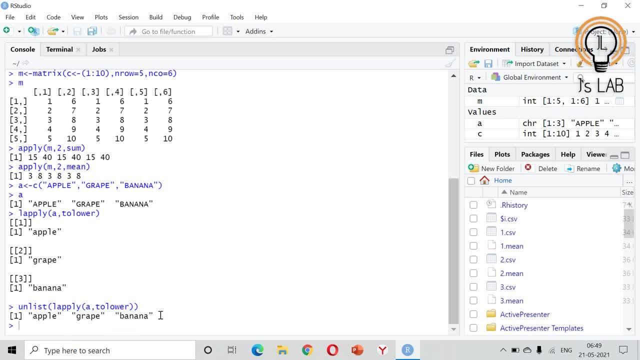 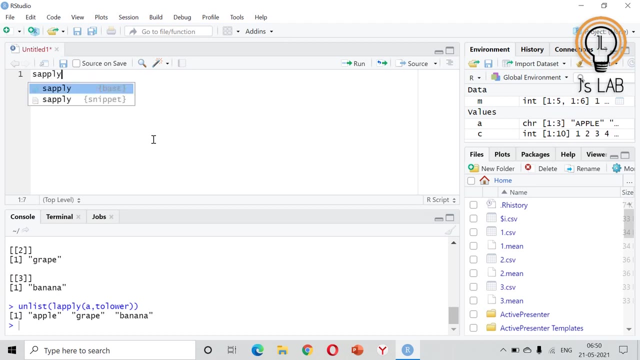 you got it as a list. your output also will be a list. input and output are list. okay, so this is L apply function. next is s apply function. so s apply is having a same arguments. s apply will have same arguments, see a function, and X is the input, a vector or an object and function. 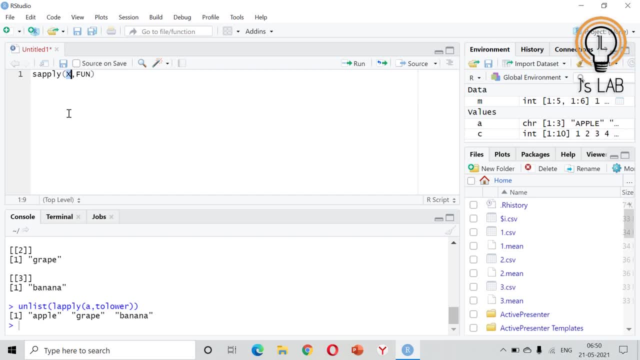 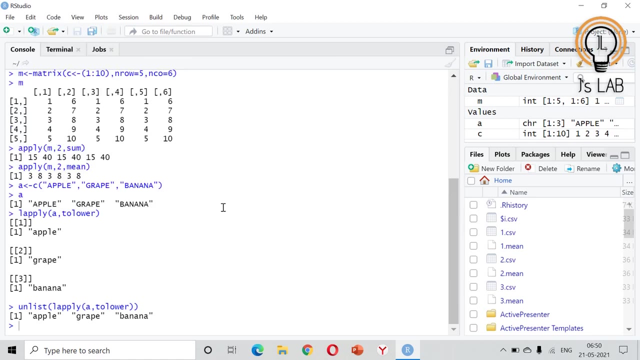 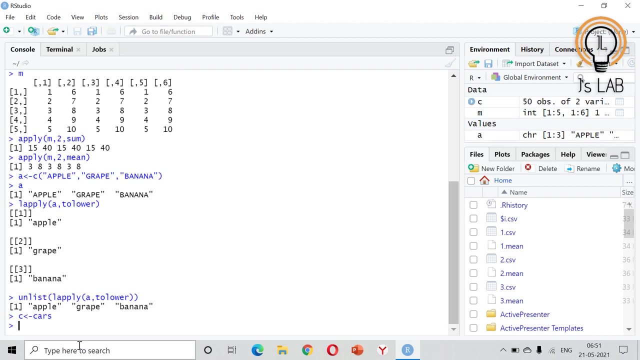 is the function that you need to apply on each element. okay, but the difference is that you will get the output also as list. okay, in the case of L, apply, you need to go for unlist function to get the output as a list. in this case, we will see cars. this is the data frame inside the R and we will print. 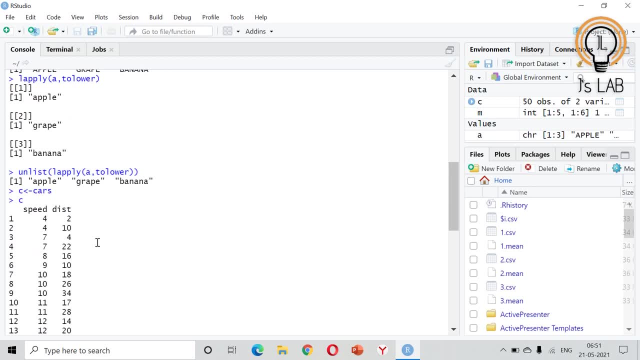 out the C. so this is the data. that means it is a data sheet with speed and distance of a car. guess, we ran distance. so you can use this data frame for a supply, supply example. so a supply. I'm going to apply it, so s apply. 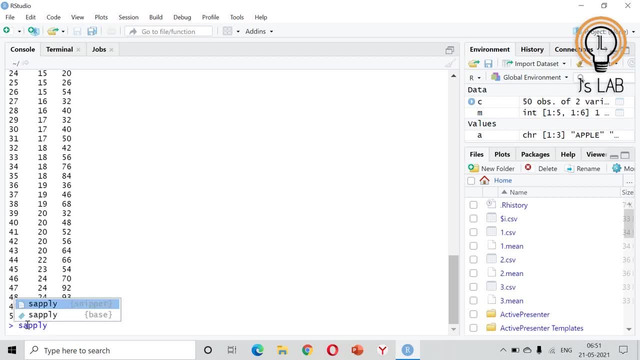 sorry, yes, apply. the input is C and I'll take max as the function. so you print C 25 and 120. so in in the, in the speed column 25 is the maximum value. in the distance, column 120 is the maximum value. it has been displayed. the same can be. 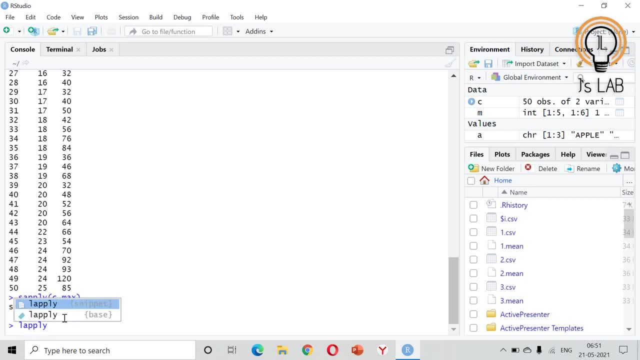 applied to L apply also, L apply C max, but it will not be in the form of a list, okay, so we need to convert that one to list. that is a small difference between L apply and s apply. now I already told you you can create your own function as well. other than this, 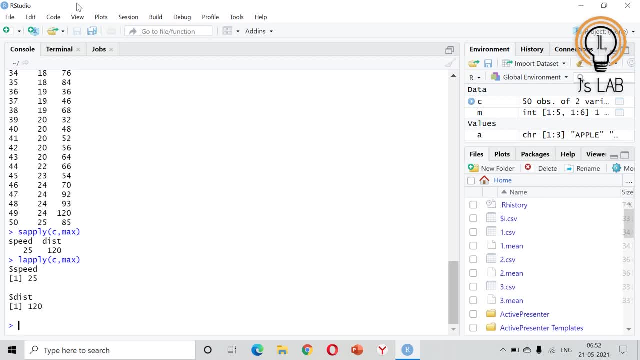 maximum, minimum, mean, mod, etc. for example, we will create average. I am creating a function- average, okay, function of X- in which what I require is I will find the X means it is the values in the data frame. I will take the minimum of X and I will add it with the maximum of X, then I will take the average away to 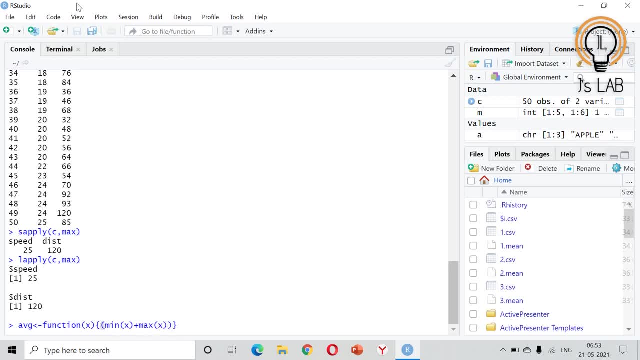 take a divided by 2. that is my required function, so I created my own customized function. okay, now I will apply the s apply s apply. s apply to X. sorry, not X. you see, that is the cars data in which i am apply. i am going to apply avg. say, it will print 14.5 and 61. so what it will? 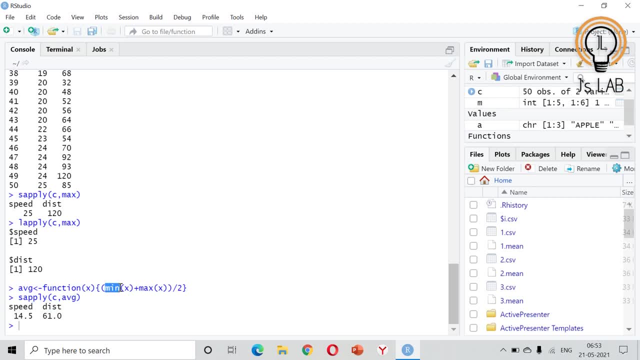 do is it will go to speed column and it will take the minimum and maximum value and it and you add and divided by 2, and it will be displayed. same thing happens to the distance column as well. so the same thing you can apply for l, apply also so this one. this is how you can create your own. 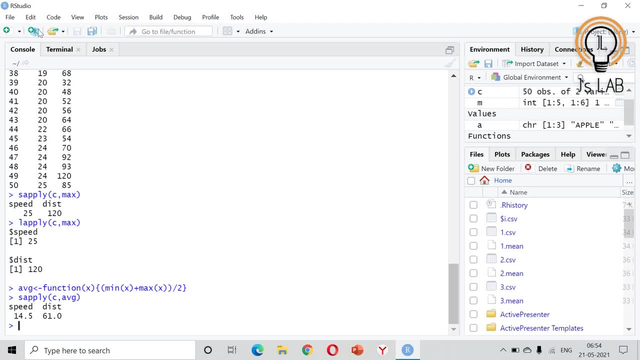 functions. now we will see the t apply function in t apply function. t apply function, you have the x. that is the input, an object, it's usually a vector. then index- index means a list containing the factor. i will show you with an example list containing factor, so on which, based on that factor, you need to do the analysis then. 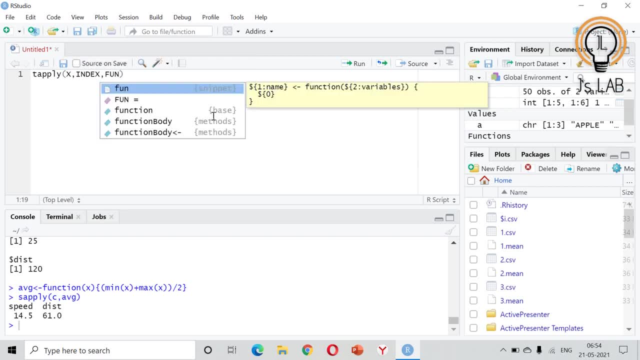 function. functions means it is a function that you that that should be entered. that means it will be applied to each elements in the vector x. it can be mean mod sum, which is available already built-in functions, or you can create your own functions, as we have discussed just before. 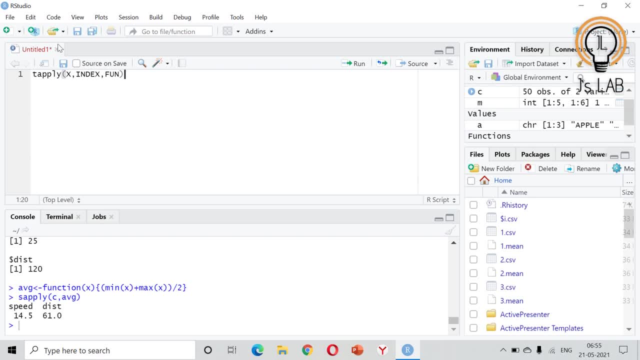 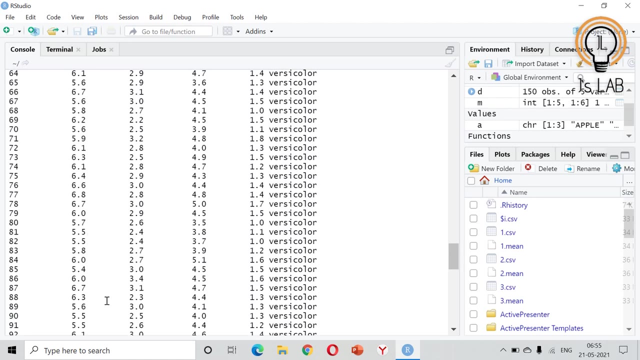 okay, so we will see an example of this. one of the t apply for that. i am taking a data set in our programming. okay, built data set. so that is iris. so if i print that one, you can see this one iris flower data. so you have the sepal length, sepal width, petal width and petal. 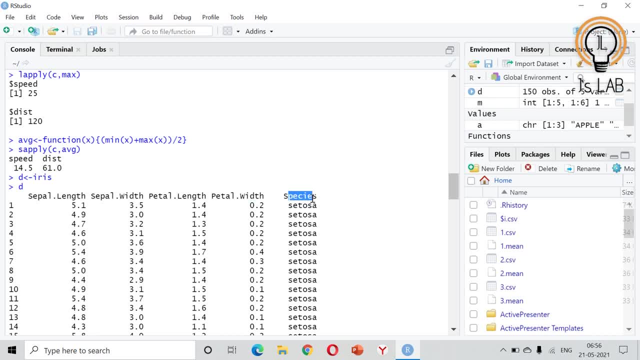 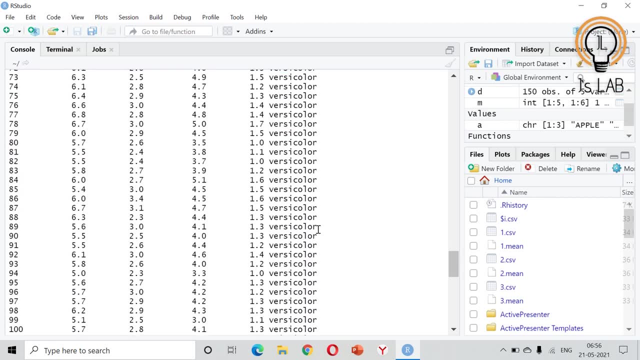 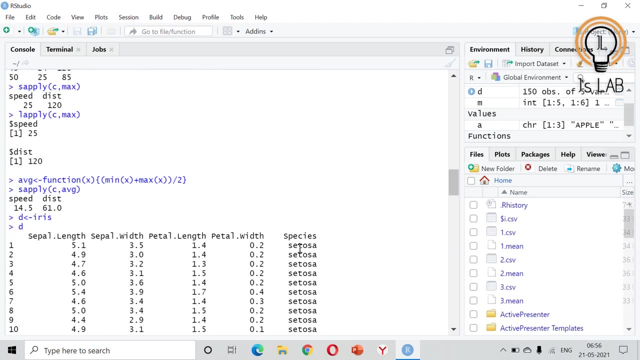 width, petal length and the species. so this is also called as fisher's iris data. so you can see, this is all about the species setosa- then you have versicolor, then you have virginica, etc. and what we need is we are going to apply t apply to this data set such that i need see, i am going to take this. 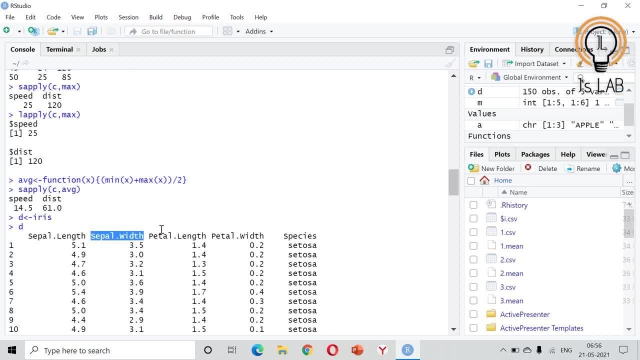 column, sepal, dot width. and for factor i am giving the species, okay, and the i am going to find the media. so what i am going to do is i need to find the median of each species of this data set. so what i am going to do is i need to find the median of each species. 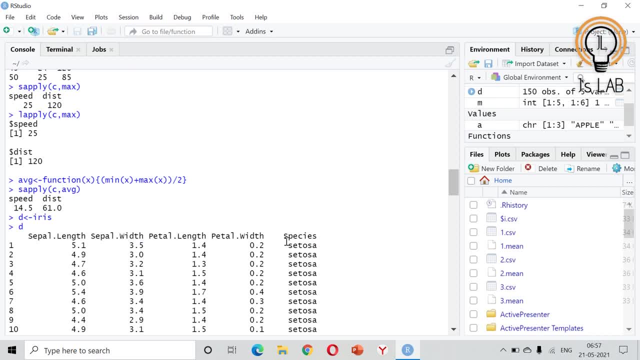 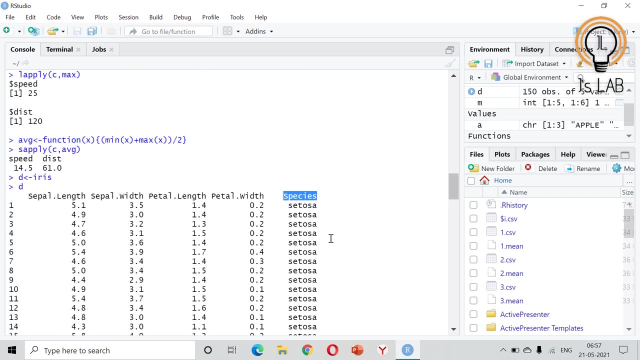 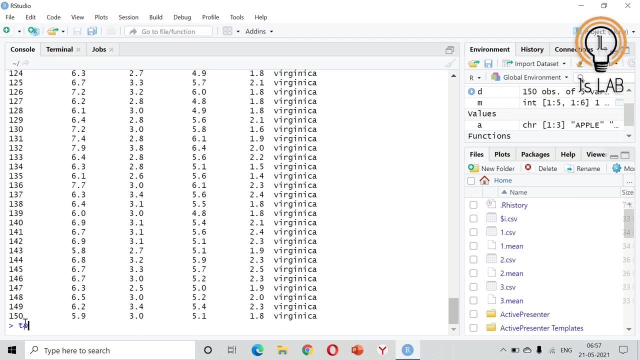 of sepal width. i need to find the median of sepal width of each species and want to display. so there are how many other- setosa, versicolor and virginica. so for each set of species, what is the sepal width? that is what we are going to find. for that we will apply t apply. t apply. our data set is d name d. 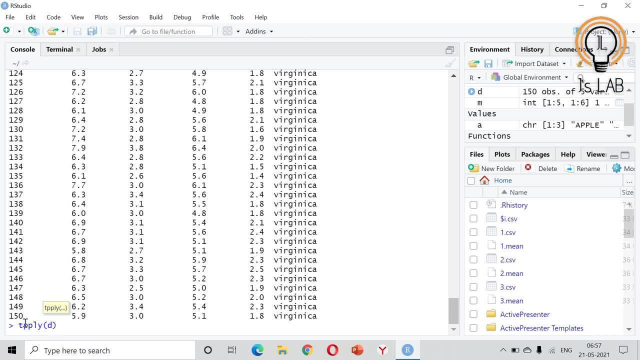 and inside d, not d. okay, you should. you need to provide inside d which one sepal width and what is the factor that is d in the d data frame, the column species. that is the factor and what is the function. i need to find the median median. so 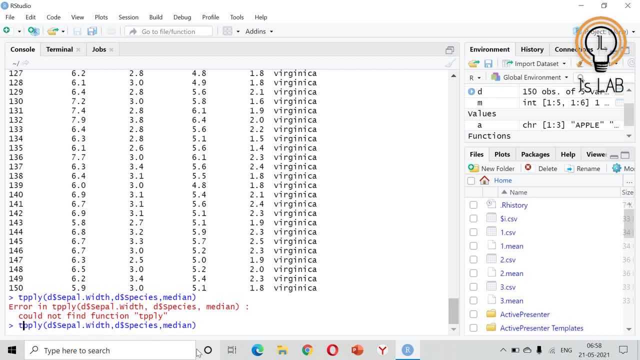 sorry, i made a spelling mistake. a is missing. okay, so here we can see setosa versicolor and virginica- three species and their sepal width medians. okay, sepal width medians. so we'll make another one. instead of sepal width, you can go for sepal length. 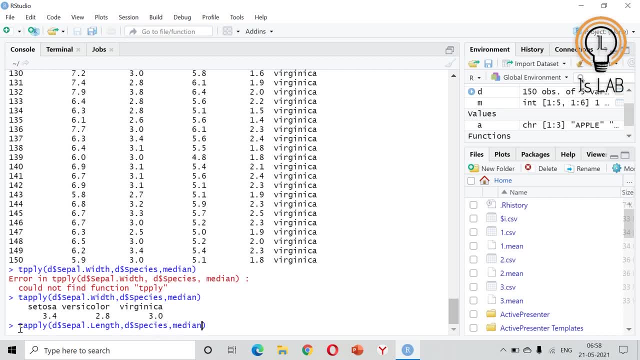 sepal length these species and we will find the maximum values. okay, so three species and its maximum values are displayed among the sepal length, so this is t apply. so we have seen the apply functions in our protein. that means apply, l apply, s apply and t apply where you can easily deals with data, frames, metrics, vectors and list. 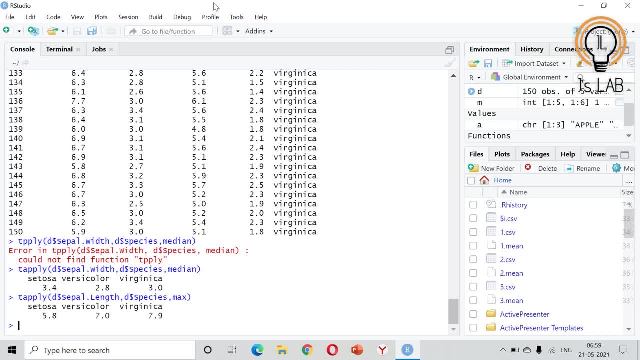 so whenever you are doing data analysis using r, this apply function is going to be a very handy tool. with just one arguments, you can apply the function to the entire data frames. the next video will be about slicing the vector using s apply and l apply method. so if you have any comments,